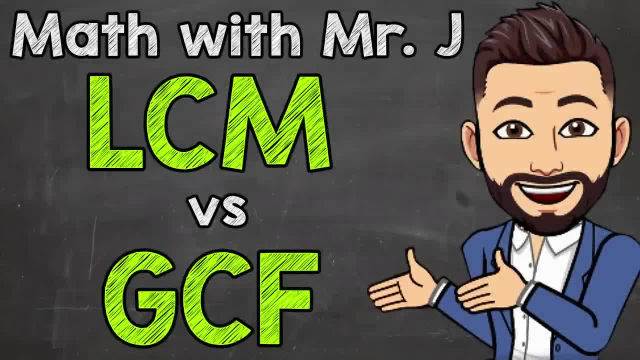 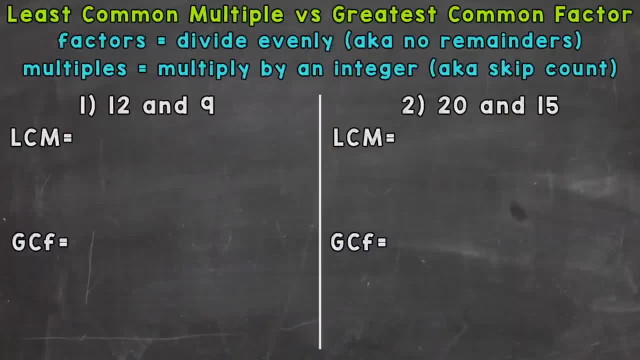 Welcome to Math with Mr J. In this video I'm going to cover the difference between greatest common factors and least common multiples. I do want to mention before I start with this, that I have a video that goes more in depth about multiples and factors. if you need more clarification on those, That link is. 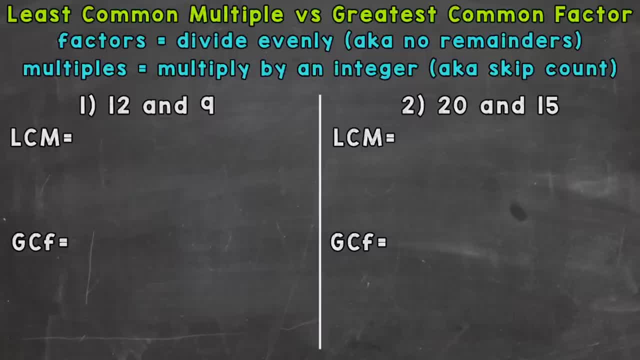 down in the description For this video. we have two examples that we're going to go through together. in order to get this down, Let's jump right into number one, where we have 12 and 9.. We'll start with the LCM, which stands for least common multiple. We'll need to write out the 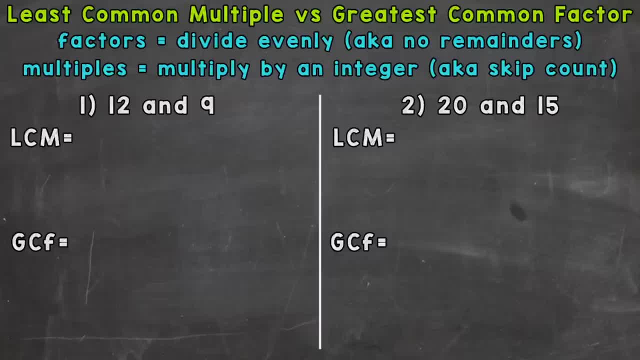 multiples of 12 and 9.. We'll start with 12.. Remember multiples. we need to multiply by integers in order to see what the multiples of 12 are. We could do this by skip counting, so we can think: Well, 12 times 1 is 12, times 2 is 24, times 3 is 36, times 4 is 48, and times 5 is 60.. 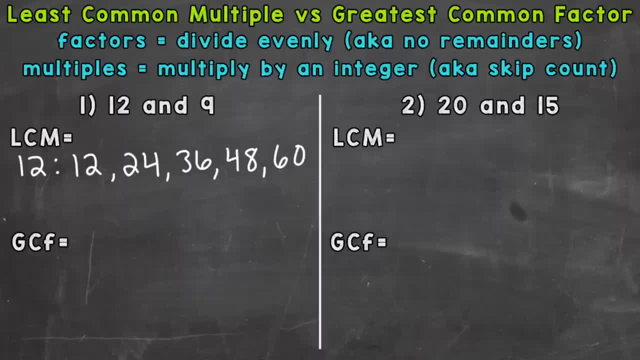 That's a good start there. If we start with four or five multiples, you don't need to do much more than that, because multiples do go on forever. You just need to start your list, do the other number and see if you have any in common. Think about what least common multiple means. 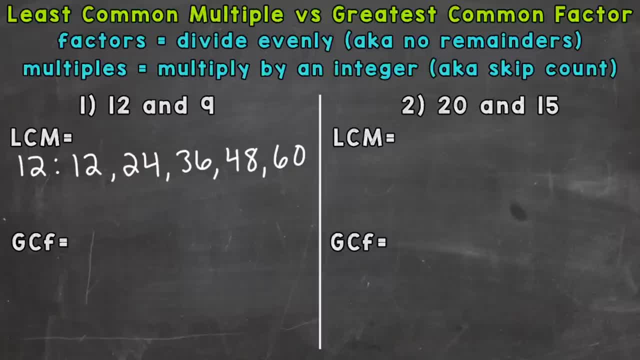 We take a look at the multiples and we find the least valued multiple that they have in common or share. Let's do 9 now and see if we have any. that match 9 times 1 is 9,, 2 is 18,, 3 is 27,, 36, and 45. Do we have any common multiples or do we need to? 3 times 1 is 26,, 4 is 65, and no, not all of them appear in common As a view. easy peasy could work like the other way. Lets move on. Let's set 32 units and the other unit to. 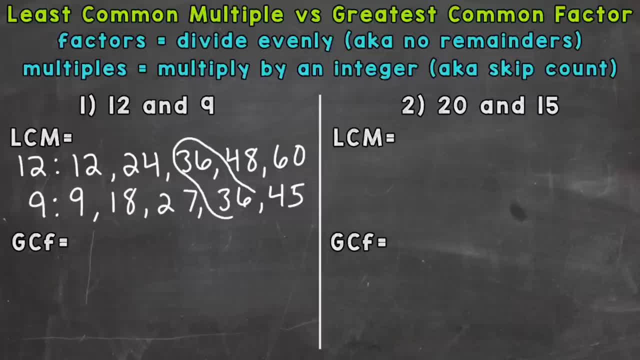 break how many. I see 26 is 36 in common. We want the least. so is there anything smaller in value that both of those multiple lists share? No. The LCM for least common multiple was 36.. Greatest Common Factor between 12 and 9. 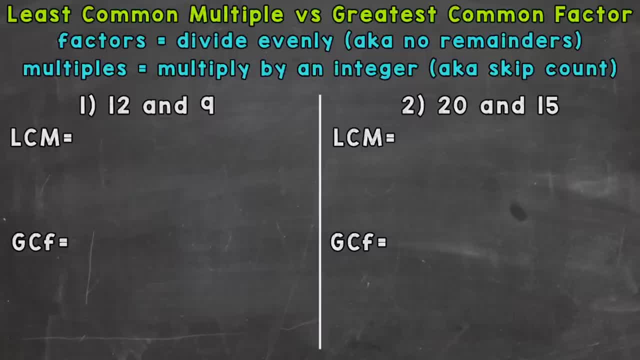 down in the description For this video. we have two examples that we're going to go through together. in order to get this down, Let's jump right into number one, where we have 12 and 9.. We'll start with the LCM, which stands for least common multiple. We'll need to write out the 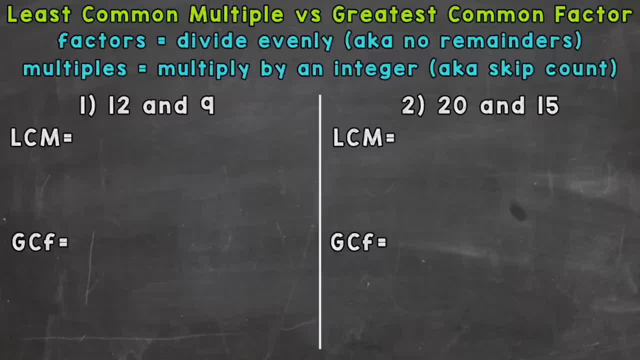 multiples of 12 and 9.. We'll start with 12.. Remember multiples: we need to multiply by integers in order to see what the multiples of 12 are. We could do this by skip counting, so we can think Let's go back to the last example and we're going to go to our first example. 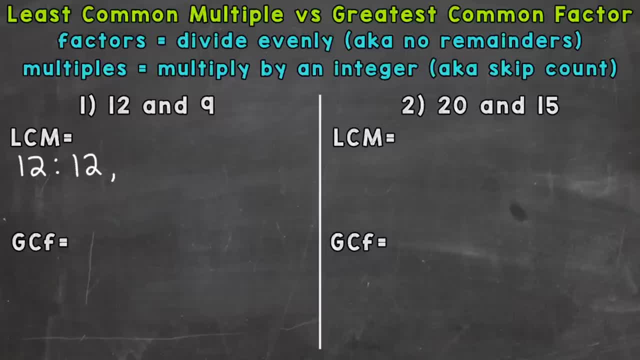 well, 12 times 1 is 12, times 2 is 24, times 3 is 36, times 4 is 48, and times 5 is 60. That's a good start there. If we start with you know 4 or 5 multiples, you don't need to do much. 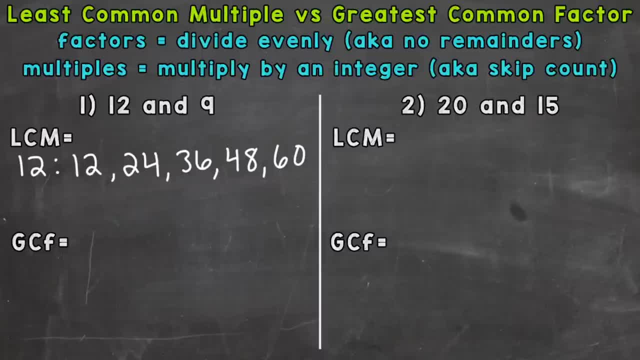 more than that, because multiples do go on forever, So you just need to start your list, do the other number and see if you have any in common. Think about what least common multiple means. We take a look at the multiples and we find the least valued multiple that they have in common or share. 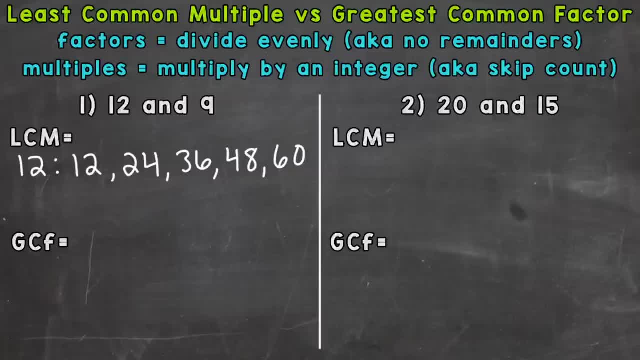 So let's do 9 now and see if we have any that match. So, 9 times 1 is 9,, 2 is 18,, 3 is 27,, 36, and 45. So do we have any common multiples or do we need to continue our list? Well, I see that we have 36. 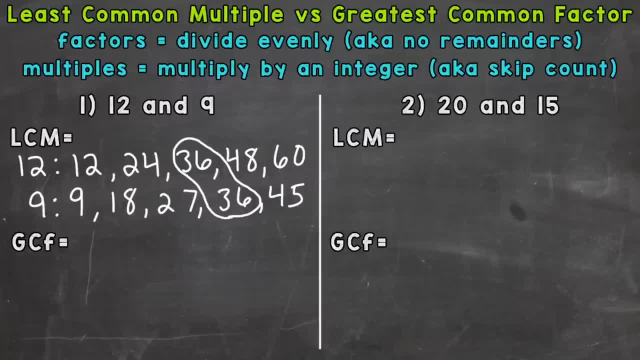 in common here, and we want the least. So is there anything smaller in value that both of those multiple lists share? No, So the LCM, or least common multiple, is going to be 36.. Let's move on to the atcher. 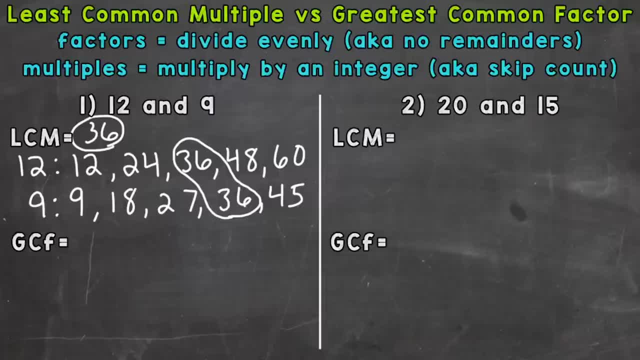 greatest common factor between 12 and 9 now, And we'll start by listing the factors of 12 and 9.. Then we need to find the greatest one that they have in common or share. Remember, factors are all the numbers that the given numbers can be divided by evenly, with no remainders, So all the RANKS IS unequivocal: RANKS ISALL llegar OR RANKS IS clinically invalid or otras. It also has more performative factors. Let's move on to the greatest common factor between 12 and 9. now We'll start by listing. 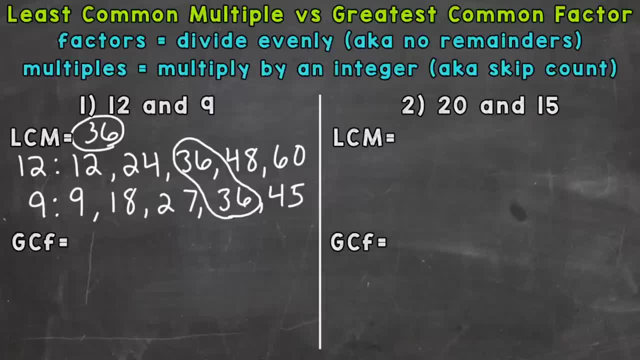 the factors with the least common factor, and then we'll start by listing the factors with the least common of 12 and 9, then we need to find the greatest one that they have in common or share. Remember, factors are all the numbers that the given numbers can be divided by evenly, with no remainders. So 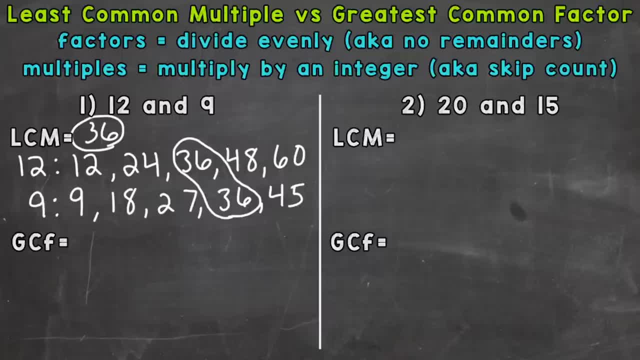 all the numbers at 12 and 9 can be divided by evenly, with no remainders. Or you can think of factors as all the numbers that can be multiplied in order to get the given numbers, So all the multiplication facts that equal 12 and 9.. I like to think of factors as all the numbers that can go. 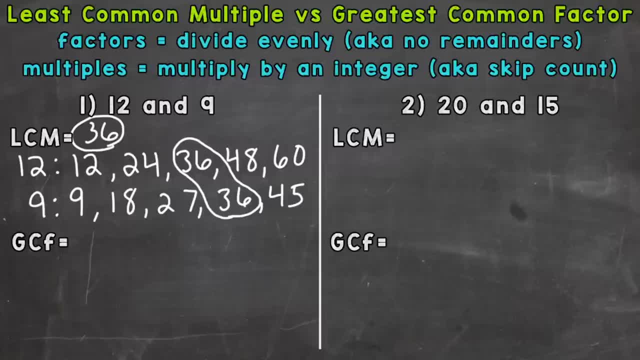 into the given number. That is not the most mathematical or technical way of thinking about it, but it helps me figure out what the factors are. when we're taking a look at greatest common factor, Let's start with 12.. So when I write my factor list, I like to start with two factors for 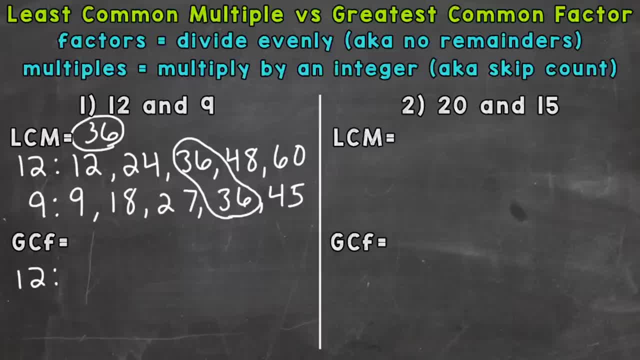 every number, And those factors are 1 and the number itself, because we know that 1 can go into 12 and 12 can go into 12.. Or, if you like to think of these as multiplication facts, that equal 12, well, 1 times. 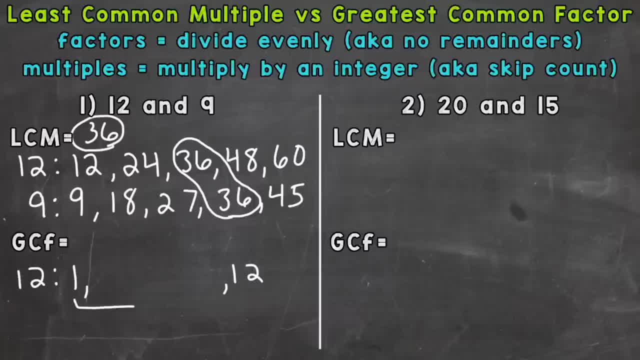 12 equals 12.. So these are a factor pair. Now I put a gap in between 1 and 12 so I can fit all the other factors or numbers that go into 12 in between there and we'll have them listed in order. 12 is even so. I know 2 is a factor. 2 can go into 12 and 2's partner is going to be 6, right? 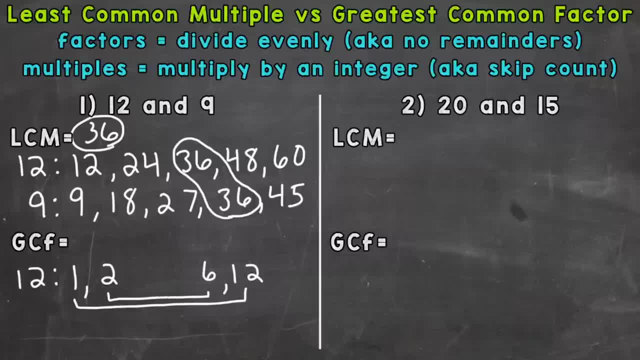 2 times 6 equals 12.. So 6 can go into 12 as well. 3 and 4 is another factor pair for 12.. 3 can go into 12 and 4 can go into 12.. Or we can think of it as 3 times 4.. 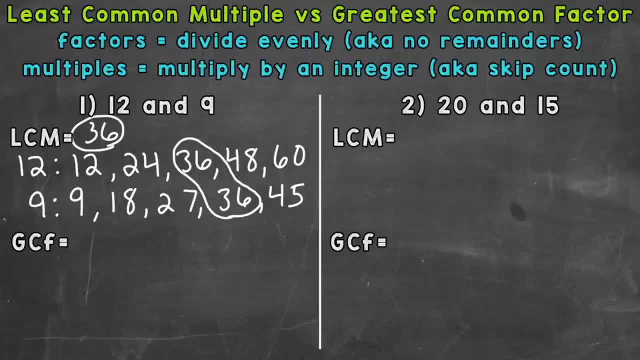 numbers at 12 and 9 can be divided by evenly, with no remainders. Or you can think of factors as all the numbers that can be multiplied in order to get the given numbers, So all the multiplication facts that equal 12 and 9.. I like to think of factors as all the numbers that can go into the 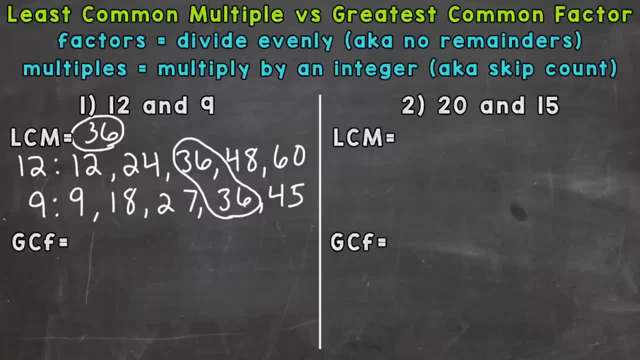 given number. That is not the most mathematical or technical way of thinking about it, but it helps me figure out what the factors are. when we're taking a look at greatest common factor, Let's start with 12.. So when we're taking a look at greatest common factor, let's start with 12.. So when we're taking a look at greatest common factor, let's start with 12.. So when 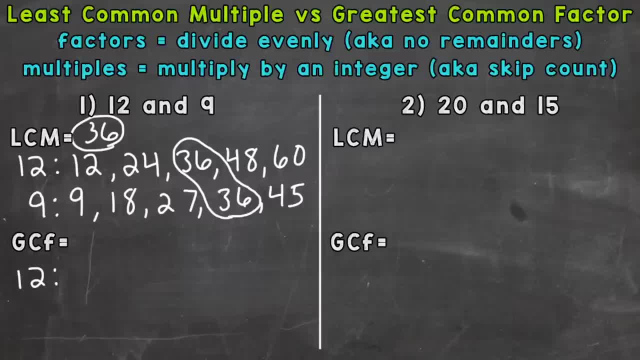 I write my factor lists. I like to start with two factors for every number, and those factors are 1 and the number itself, because we know that 1 can go into 12 and 12 can go into 12, or, if you like to think of these as multiplication. 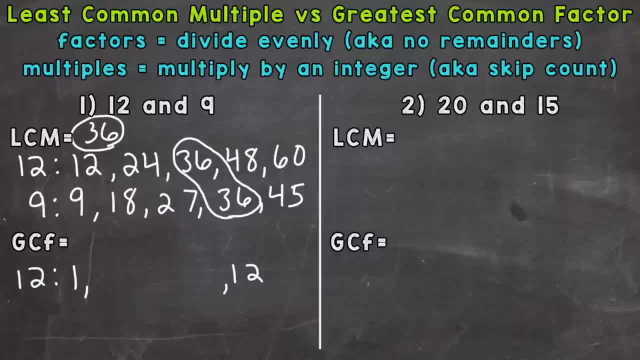 facts that equal 12. well, 1 times 12 equals 12, so these are a factor pair. now I put a gap in between 1 and 12 so I can fit all the other factors or numbers that go into 12 in between there, and we'll have them listed in order. so 12 is 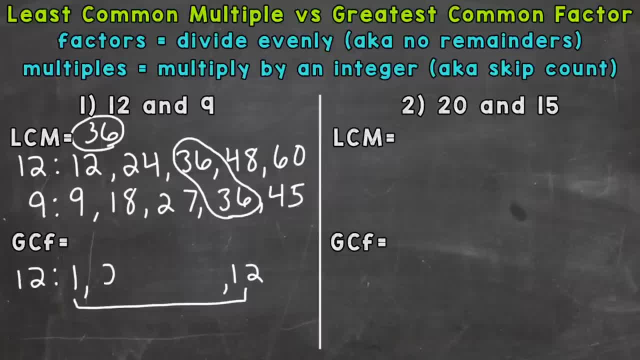 even so, I know 2 is a factor, 2 can go into 12 and 2's partner is going to be 6. right, 2 times 6 equals 12, so 6 can go into 12 as well. 3 and 4 is. 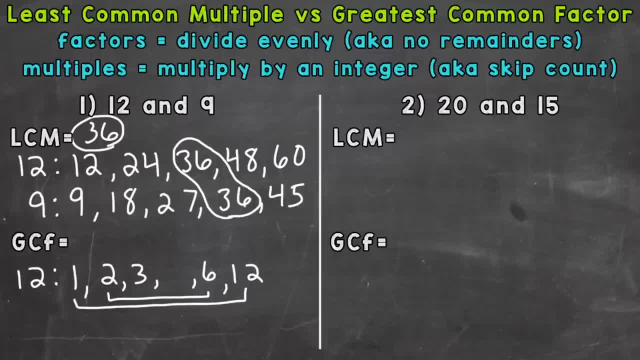 12 and 12 can go into 12 as well. 3 and 4 is another factor pair for 12. 3 can go into 12 and 4 can go into 12. or we can think of it as 3 times 4 equals 12. now those are all the factors of 12, so we can. 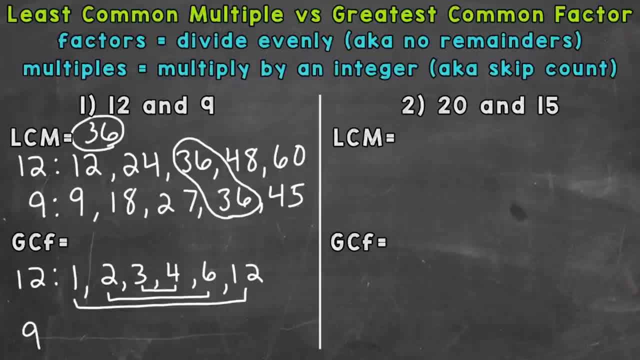 write our list for 9 now and we can start with 1 and 9, put a little gap in between and then we can list our factors. so 9 is- let me actually put, these are a pair there, so I'd like to connect them sometimes- and then 3 is also a factor. 3 times 3 equals 9. 3 can go into 9, but we 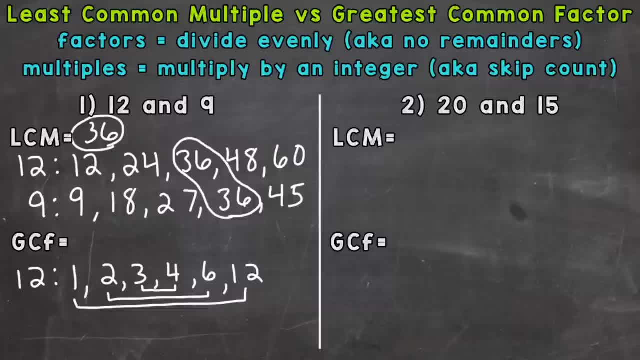 equals 12. now those are all the factors of 12. so we can write our list for 9 now and we can start with 1 and 9, put a little gap in between and then we can list our factors. so 9 is, let me actually put, these are a pair there, so I'd like 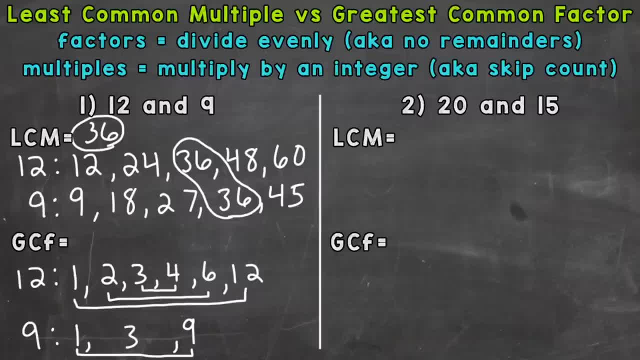 to connect them sometimes. and then 3 is also a factor. 3 times 3 equals 9, 3 can go into 9, but we only need to list 1- 3. we don't need to put 2 there. so 1, 3 and 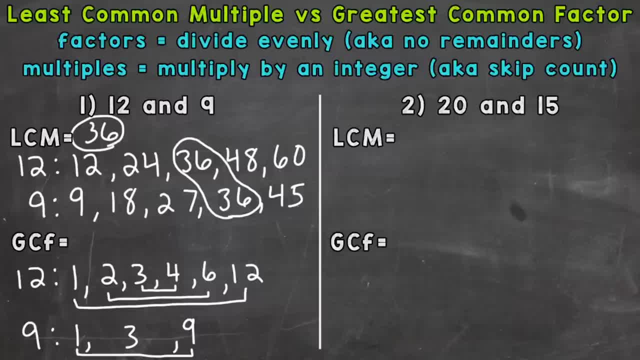 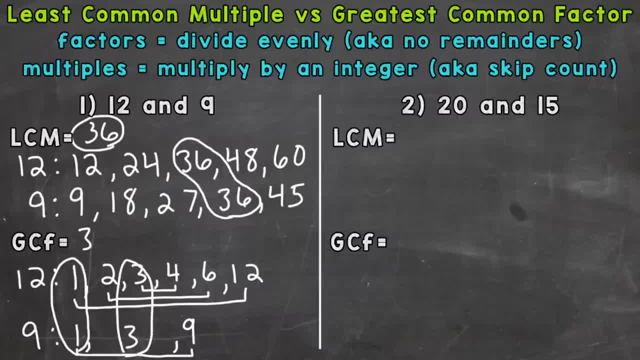 three. so 3 is going to be the greatest common factor between 12 and 9. now, as far as spacing and writing out those factor lists, you'll get much better at those the more you do, so let's move on to number 2, where we have 20 and 15. so 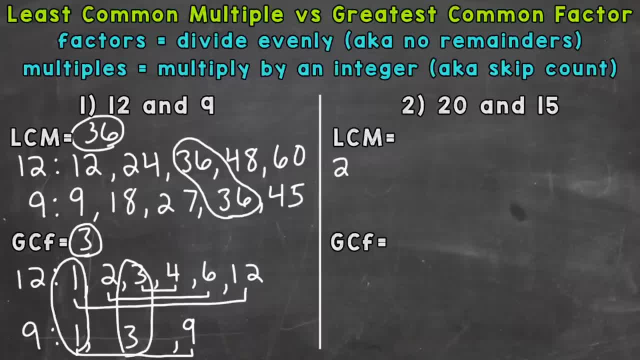 least common multiple first. so we'll write out the multiples for 20 and 15. so 20 would be 20, 60, 80, 100. so you can start your list by writing out 4, 5, seeing if you have a match. if not, you can always continue. 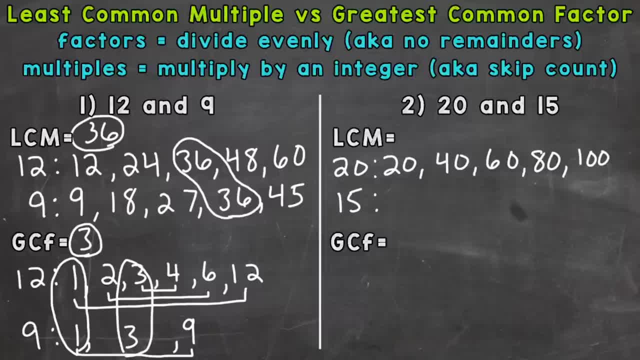 lists because, remember, multiple lists continue on forever: 15, we would do 15, 30, 45 and 60, and you'll notice that we have a match here. always double check and keep on seeing that the lists have always også continuar. ו Pskeผม immortaloneyć הтоб är 5 AND 60. und là, lевич lines, last street, 19, can be alwaysее incorrect. Catherine Quesadinhos country gibt uns aucalled les uppermăng Giant's here, always don't. 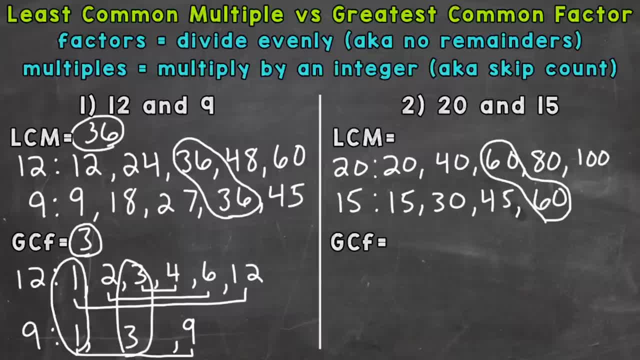 check if you have anything that is smaller in value, because, remember, least common multiple, 60 is going to be the least that they do have in common. so that's going to be our LCM, or least common multiple, greatest common factor. we will write out our factor lists for 20 and 15, so we'll start with 20 here. 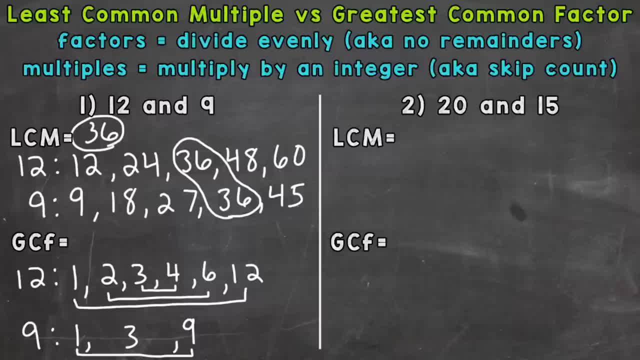 only need to list one, three. we don't need to put two there. so one, three and nine are the factors of nine. so once we have those lists of factors, we find the greatest one that both those lists share what they have in common. so we can see: 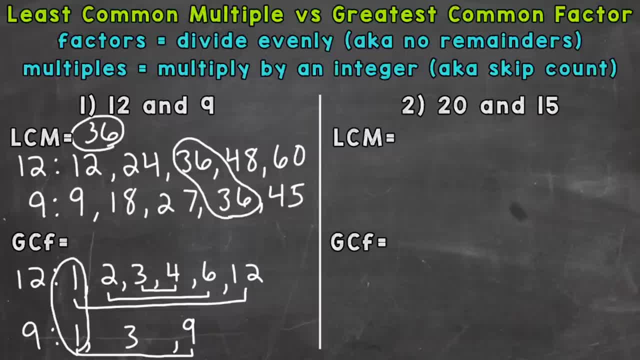 that they are the list of factors that we need to put into 9 and we can list the have one in common, but we want the greatest, so anything greater. yes, three. so three is going to be the greatest common factor between twelve and nine. now, as far as spacing and writing out those factor lists, you'll get much. 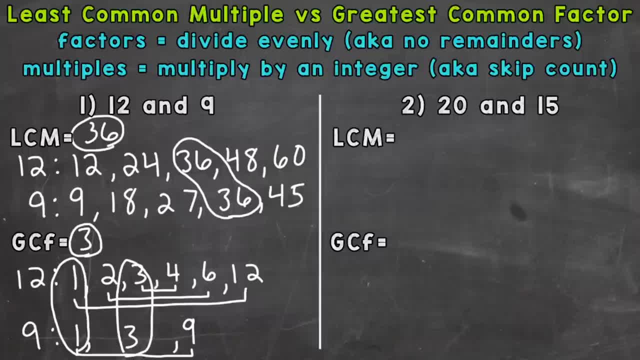 better at those, the more you do. so let's move on to number two, where we have twenty and fifteen, so least common multiple first. so we'll write out the multiples for twenty and fifteen. so twenty would be twenty, forty, sixty, eighty, one hundred. so you can start your list by writing out four or five, seeing if you have a. 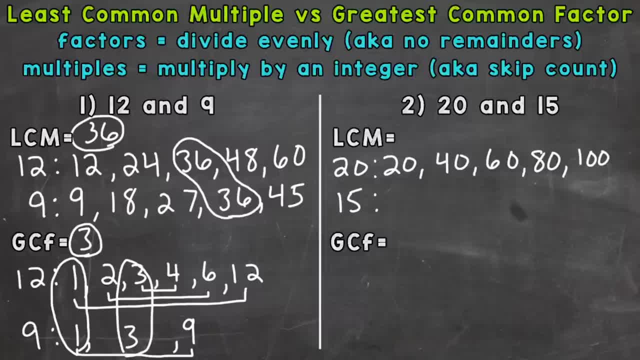 match. if not, you can always continue lists because, remember, multiple lists continue on forever: 15, we would do 15, 30, 45 and nine And 60 and you'll notice that we have a match here. Always double check if you have anything that is smaller in value, because remember least. 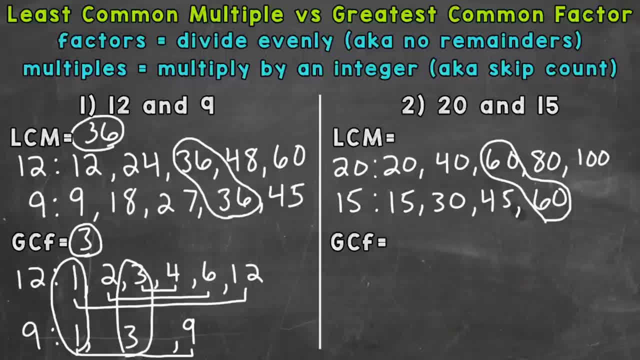 common multiple, 60 is going to be the least that they do have in common. so that's going to be our LCM or least common multiple, Greatest common factor. We will write out our factor lists for 20 and 15.. So we'll start with 20 here and 1 and 20.. 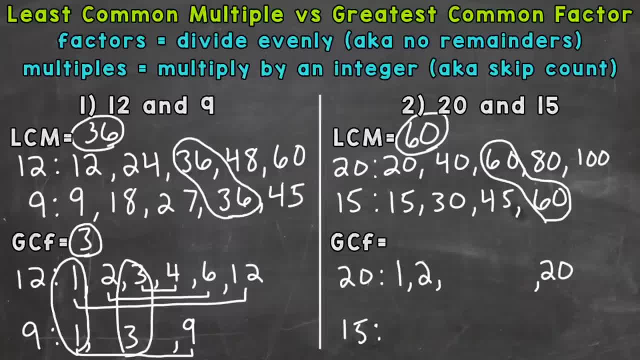 We know that 2 can go into 20, because 20 is even and 2's factor pair here, or partner, is 10.. We also know 4 times 5 equals 20, or we can do 20 divided by 4.. However you like to think of it. 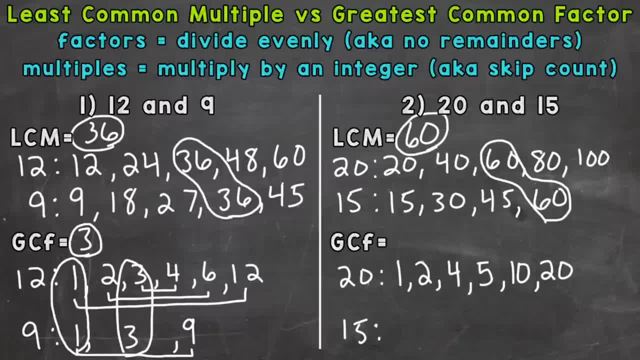 So we know that 4 and 5 are also factors of 20.. So those are all the factors of 20.. Now we need to list the factors of 15.. So we'll start with 1 and 15, and then we also know 3 and 5 are factors of 15..